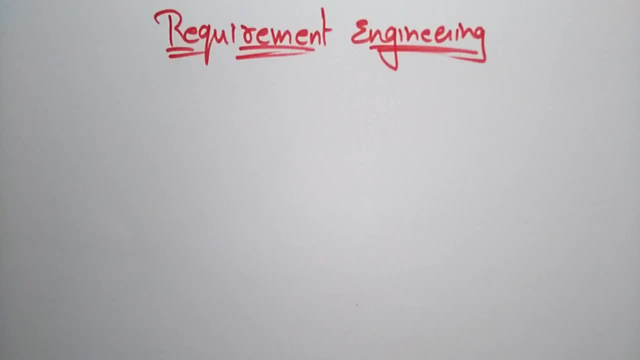 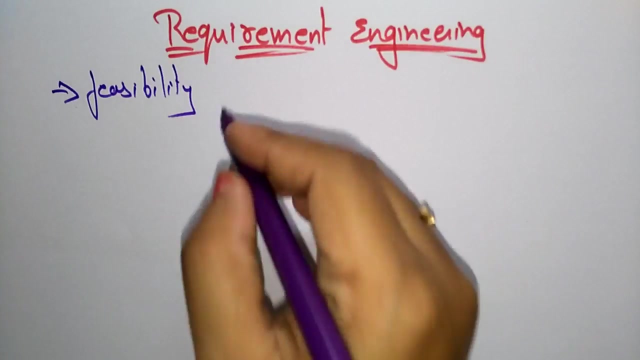 Hi students. now coming to the next topic, that is, the requirement engineering. So what are the requirements for the engineering to develop any product? So the requirement engineering has to think about the feasibility study. So after developing the SRS document, that is the software requirement specification, So this is a foundation for the product or a project. So there, first you have to think about the feasibility study. 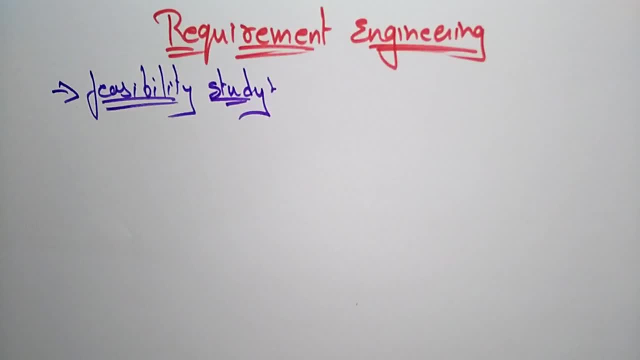 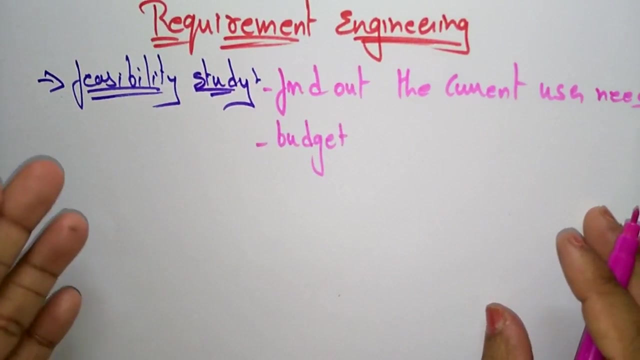 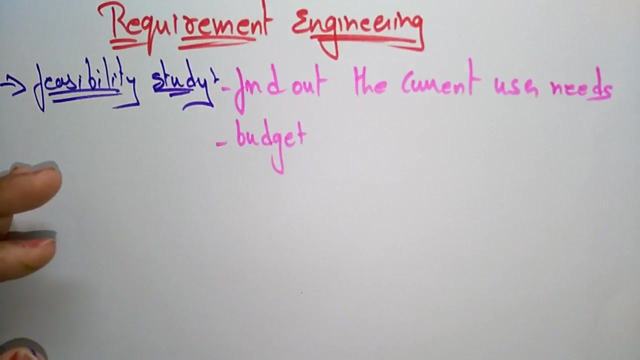 The feasibility study here is it find out the current user. So current is a user needs and budget. So in the feasible study, the requirement engineering going to be study about the find out the current user need, what exactly the current user needs and what is a budget is going to be given to that project. 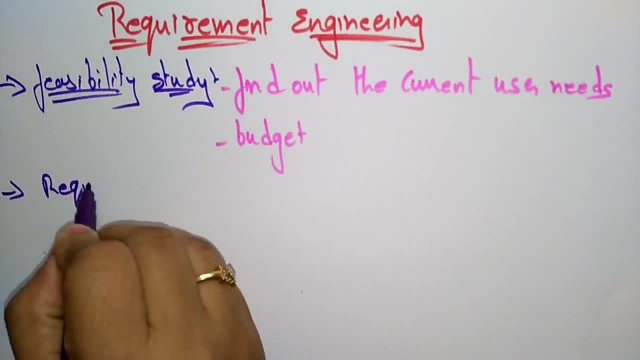 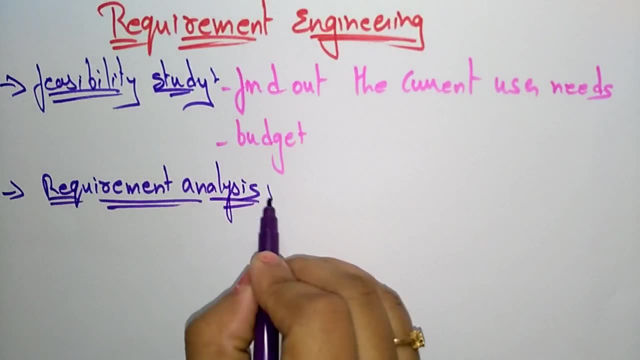 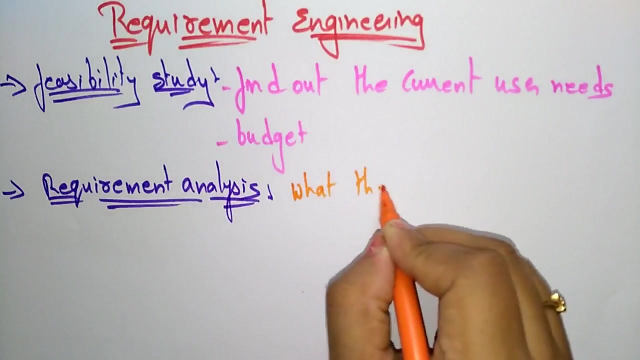 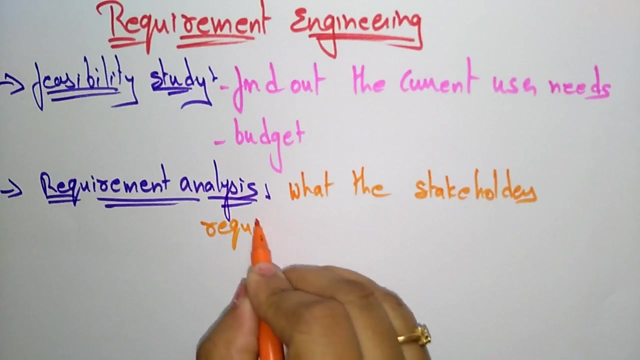 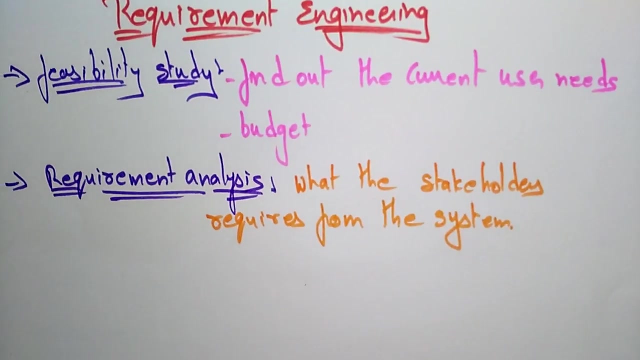 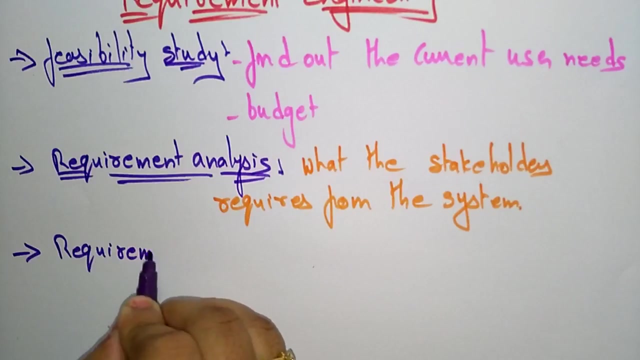 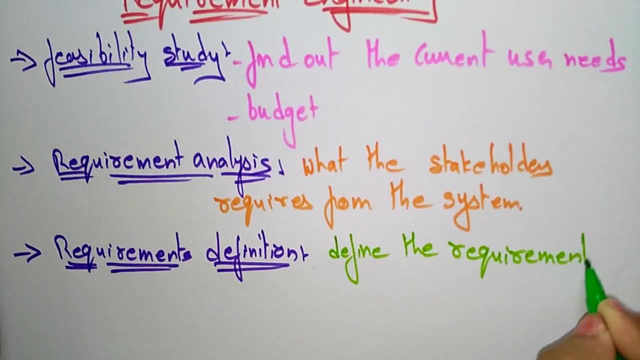 Next, requirement analysis. So in the requirement analysis they have to think about what the stack holder, what the stack holders requires from the system, what exactly they want requires from the system. and next, requirements definition. So requirement definition is nothing but it defines the. it define the requirements in the form of, in the form understandable to the customer. 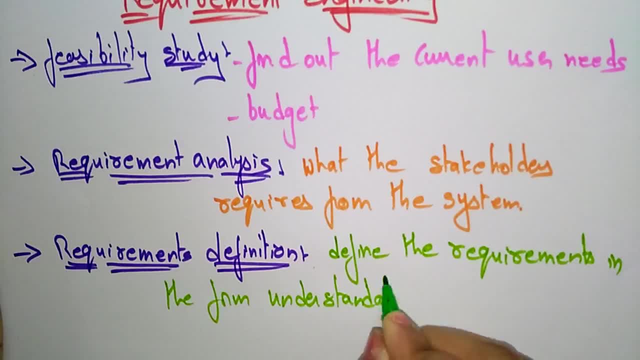 And it defines the. it defines the устandable to the customer. So the main aim of here is to developing the requirements. engineering is requirement definition, So it has to be some clear-cut view about the project. What is they are going to be developed by taking the requirements from the customer.